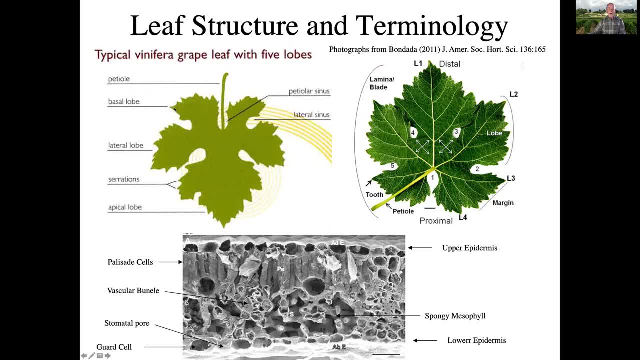 blade And these leaf blades are sometimes completely round but in other cases have lobes on them and different numbers of lobes, And they have these indentations which are called sinuses. So we have a petiole or sinus right near where the petiole attaches, And this is often 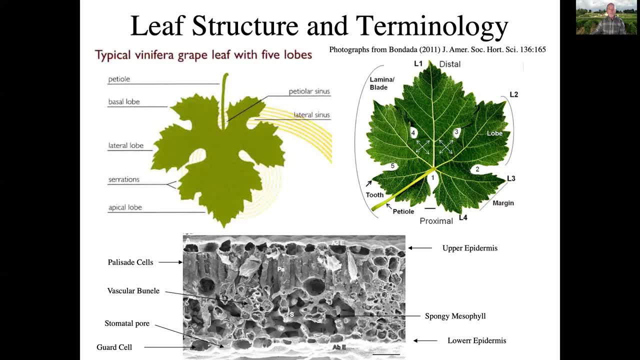 a very significant identification mark on the terms of the way the shape is. It could be a U-shape, as in this case, or it could be a V-shape or even flatter. We have these lateral sinuses as well, So we count the number of lobes. 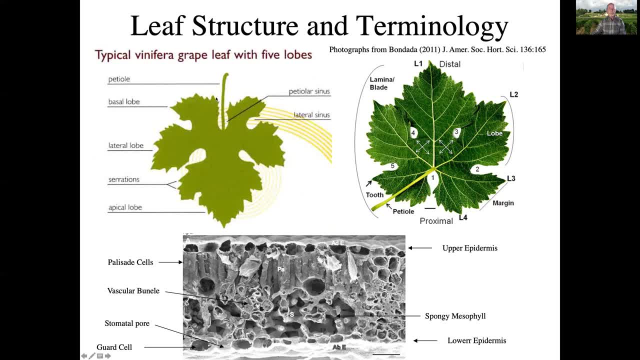 And then the other particular characteristic that's important is the margin of the leaf. Sometimes those leaves are smooth, Sometimes they're known as teeth, as in this picture here of a Merlot grape leaf, Or sometimes they're deeper, more serrated. So these are. 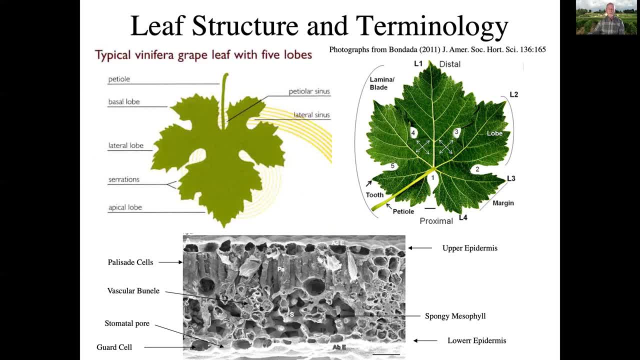 the characteristics or attributes that you're looking for when you're trying to identify a grape variety. The leaf venation is also quite striking And you can see that these veins go quite a ways all throughout the leaf and ultimately close to all the plant cells. 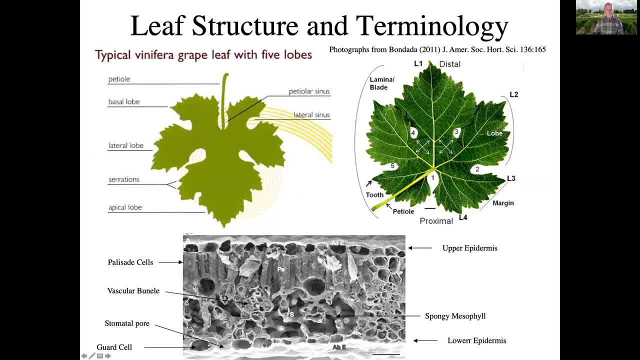 So here's a cross section of a leaf just to give you an idea of what a grape leaf is like. We have a upper epidermal layer here that is completely closed off, whereas we have a lower epidermal layer here where we have our stomates, the stomatal pores, which 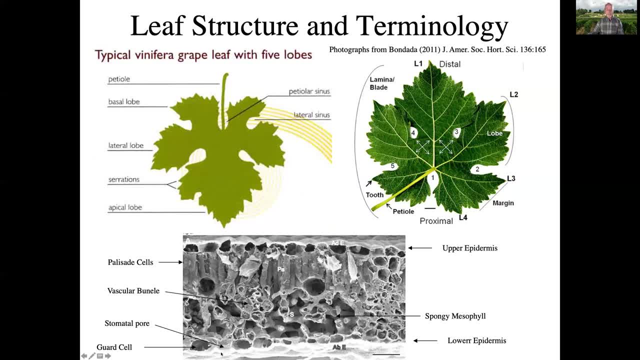 open and close and let CO2 into the leaf and water outside the leaf. This is controlled by the guard cell, So we only have stomatal pores on the lower epidermis of the leaf or the abaxial side of the leaf. We have additional cell types in here. 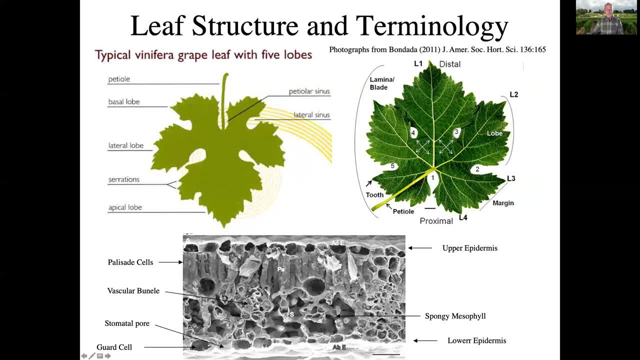 This is the palisade cells. These are dense cells where most of the photosynthesis is going on. Very little is going on in the epidermal layer, And we have another type of photosynthetic cell called the spongy mesophyll cells. These are much more loosely packed so that the CO2 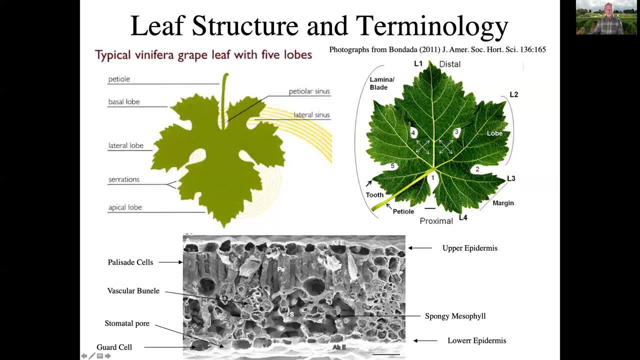 can diffuse into these air spaces and photosynthesis can occur. And then right here we see which is hard to make out in this cross section, but it's vascular tissue. That is the xylem and phloem piping is coming in from below through the 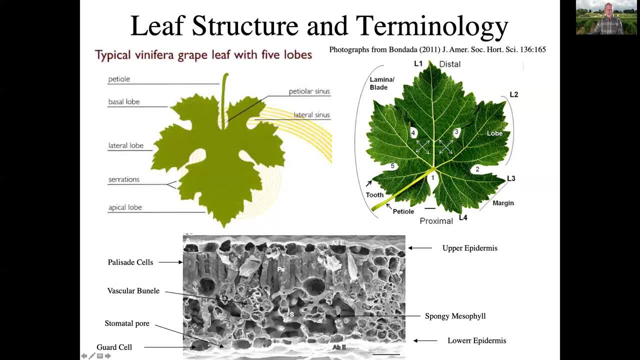 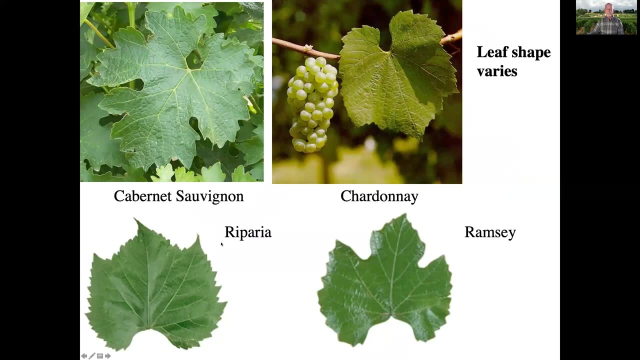 petiole to the leaf and providing water and allowing sugars from these photosynthetic cells to be pumped back out to the rest of the plant. So leaf shape varies quite a bit. You can see it here in a few examples. Here we have 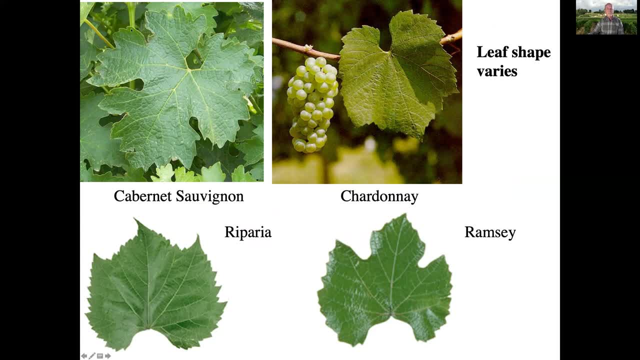 a Cabernet Sauvignon. This is a Cabernet Sauvignon leaf which has five lobes and it has deep sinuses and deep serrations. And here over here, we have the Chardonnay leaf, which has got very little. 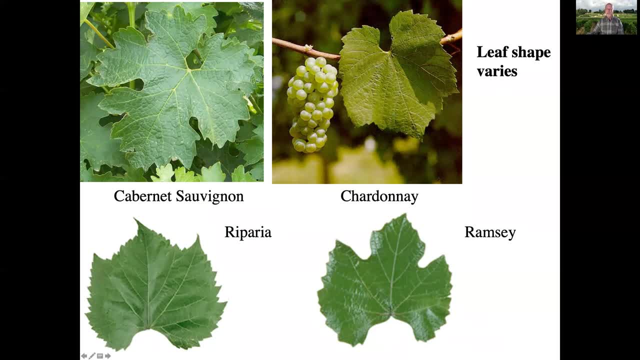 sinuses whatsoever. There's a large petiolar sinus here, but we don't have such distinct lobes. but there are lobes And you can see the margins here are more tooth-like. Here are two wild species. This is Vitis riparia, which is from the Northeastern United States, And again you 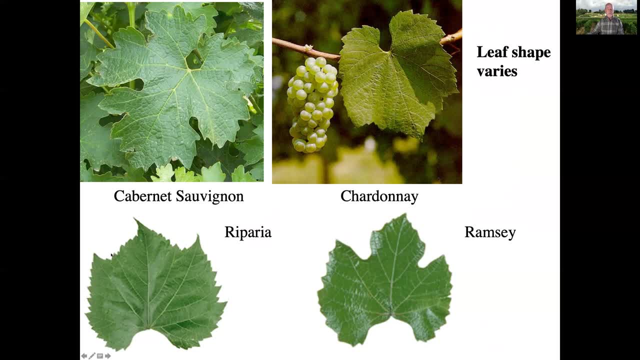 can see, the lobes are not so distinct. There are in a sense five lobes here, but very, very short. And then notice the petiolar sinus is much more open and round, And here is a Vitis. champigni, or commercially known as Ramsey comes from, originates from 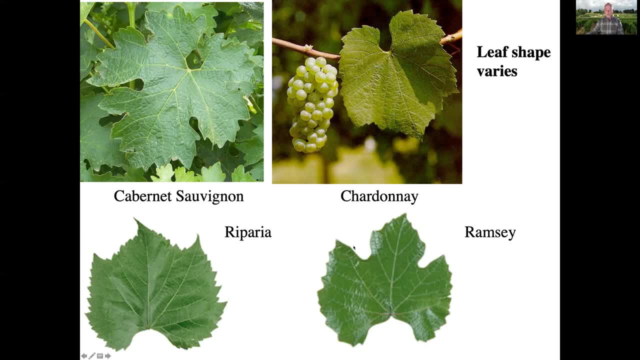 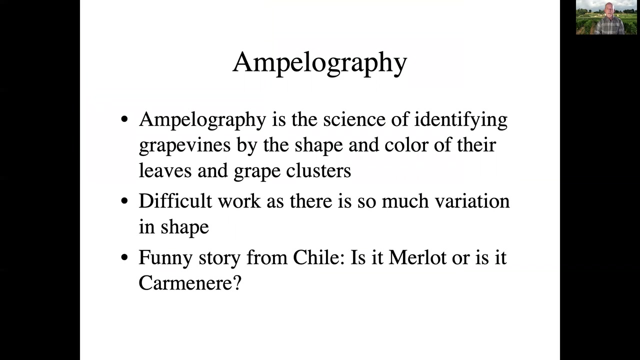 the Texas area, And you can see deeper sinuses here Again, a very distinct, almost V-shaped sinus here in the petiolar sinus. So these are ways of identifying different species as well as different cultivars. The science of identifying grapevines by leaf shape and by the color of the grape clusters. 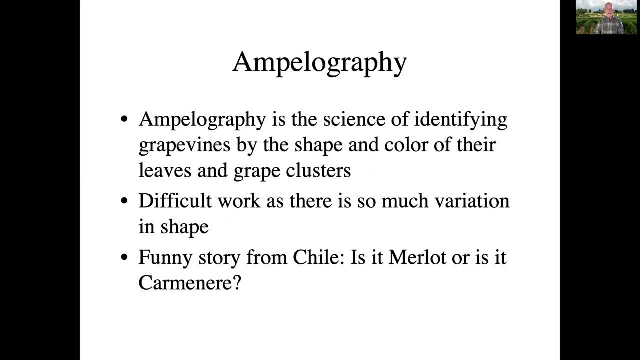 and the shape and size of the grape clusters is known as ampillography. This is a very difficult work to do because there's so much variation in varieties, in cultivars and on a single plant. You can see variation in leaf shape just on a single shoot. 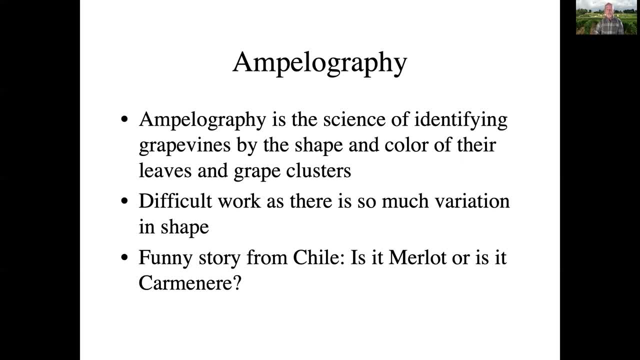 from the bottom to the top. That makes it very hard to identify. And in fact in our own vineyard we had some Pinot Blanc leaves that I began to think were Chardonnay leaves or the other way around. I guess it was. I had Chardonnay leaves that. 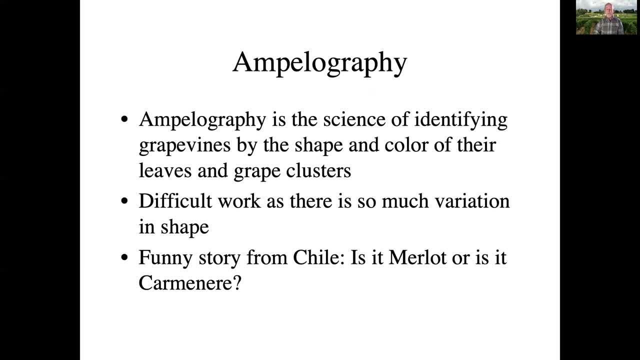 I thought looked like Pinot Blanc leaves and I wondered if there had been a misidentification. So we sent pictures down to Davis to Dr Andy Walker and he seemed to confer that it looked like Pinot Blanc leaves. He noticed a small difference in lightness and he said: 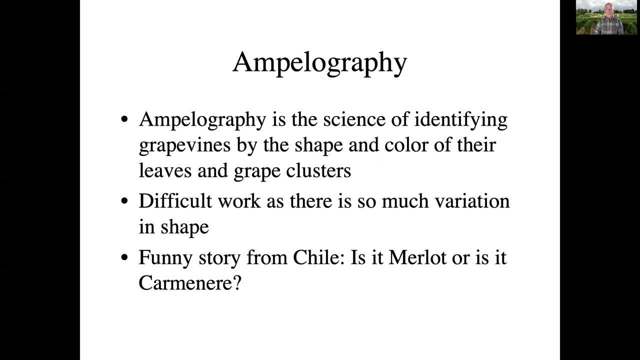 like these might actually be pinot blanc leaves rather than, then, chardonnay. so to be sure that we sent some leaf samples down where they did some DNA testing, only to find out that indeed they were chardonnay leaves. so even the experts can be fooled. and this leads me to a funny story. when I was in Chile for the 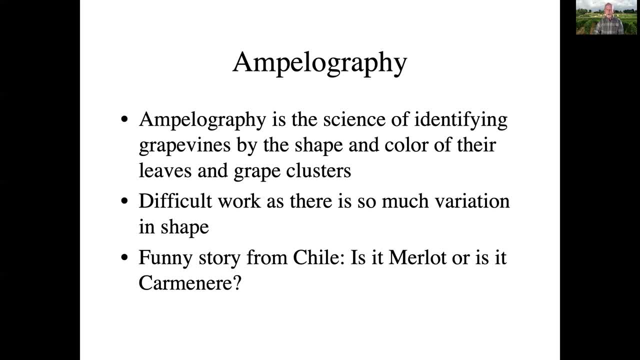 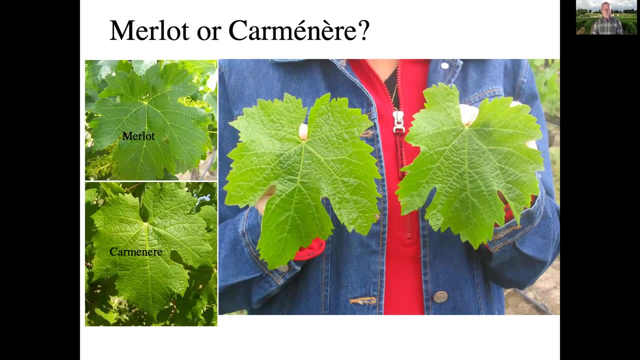 first time we were touring around Chile and my colleague down there was telling us a story about Merlot and Carmenere in Chile. so for many, many years the industry was making grapes, making wine from grapes that they called Merlot grapes, and for about 20 years they were selling it around the world as Merlot. 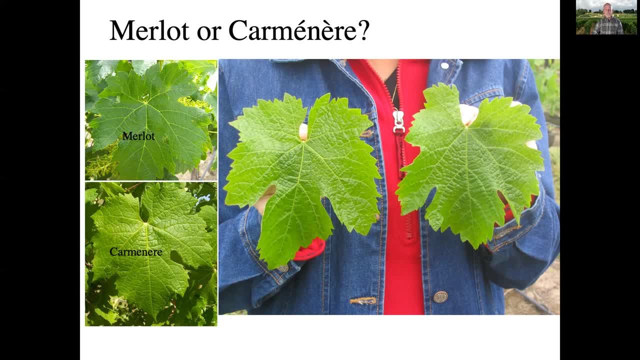 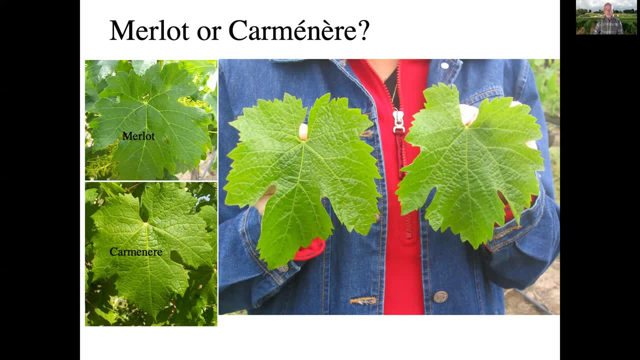 grapes and they went: well, it isn't well, what is it? and he said: I don't know. and eventually, ten years later, a another appellographer, young French appellographer, came down to identify it as Carmenere grapes, which was a very rare old French grape variety that was not growing much in France anymore. 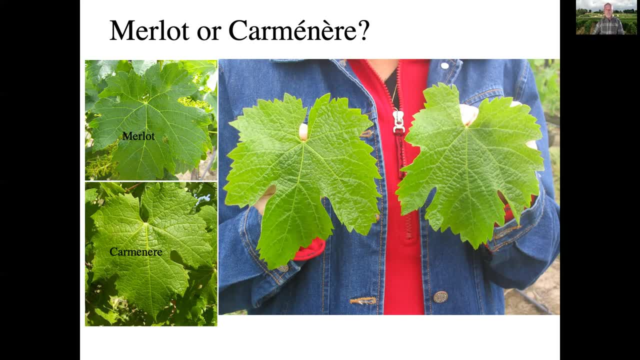 but that vineyards were large amounts of them in Chile. so now you see wine being sold pretty much only from Chile, of Carmenere. now here's an example down there on the left, up here we have Merlot leaf and down below is a Carmenere leaf, a. 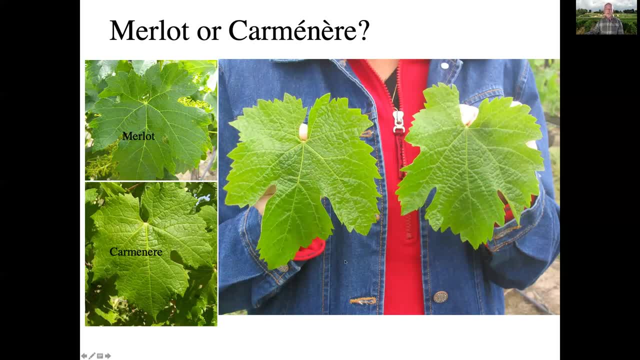 and I have my beautiful assistant here, my wife holding those leaves next to each other, and now use your training that you just had to look at the sinuses, the shape of the sinuses and the leaf margins and tell me which great leaf is Merlot and which grape leaf is Carmenere. I'll give you one second wait, just just. 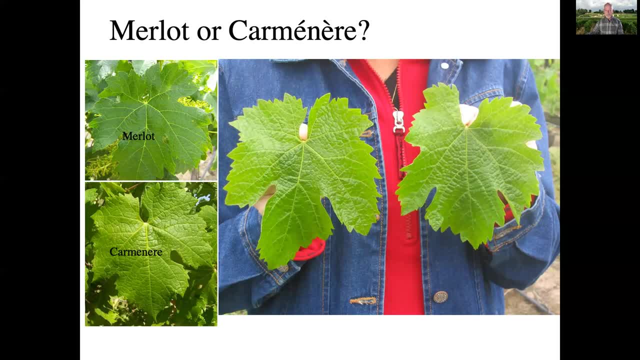 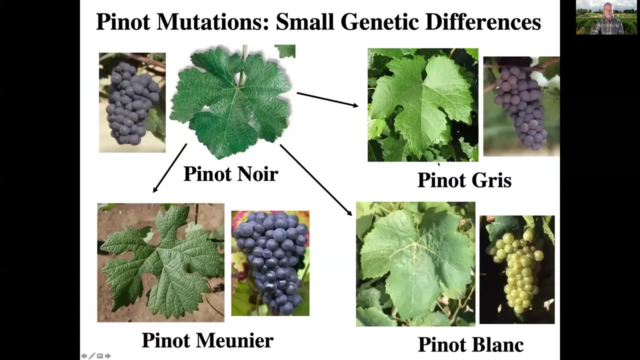 give you one second or two or three or four to decide. the answer is: the left one is Carmen Eyre and the right one was Merlot. how did you do? it's not easy, is it okay? so we're going to talk a little bit about how genetic, very small genetic. 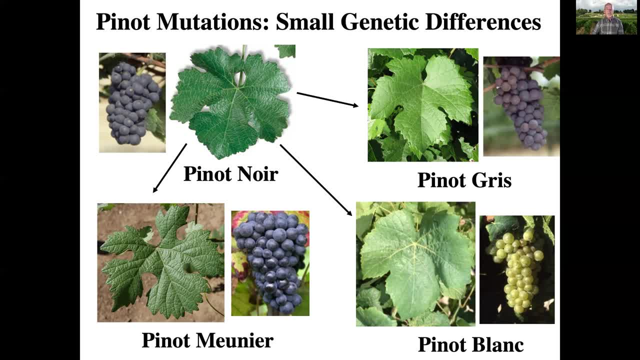 variations can make big differences in grapes. Pinot Noir is an old, old variety going back at least to 900 AD in France, and has given rise, through mutations, to a number of different genotypes, some of which we call cultivars, some of which are clones. I don't know what the difference is between a cultivar and a. 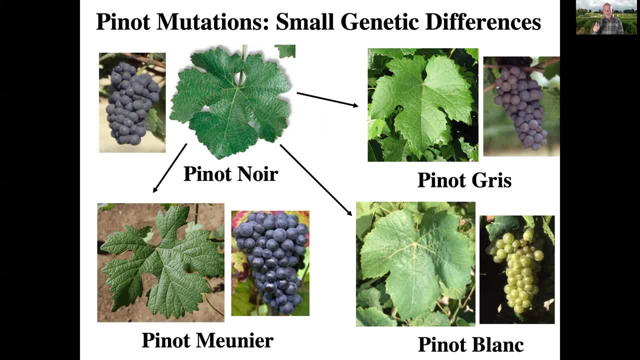 clone and how one decides that this is genetic, and how one decides that this is genetic and how one decides that this is to be a cultivar and not a clone. because to be a cultivar and not a clone, because to be a cultivar and not a clone, because, in this case, between Pinot Noir and. 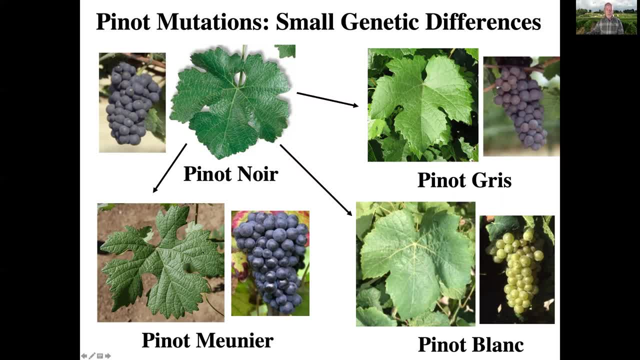 in this case, between Pinot Noir and in this case, between Pinot Noir and Pinot Meunier, it's a single gene mutation. Pinot Meunier, it's a single gene mutation. Pinot Meunier, it's a single gene mutation that causes. this is a large difference. 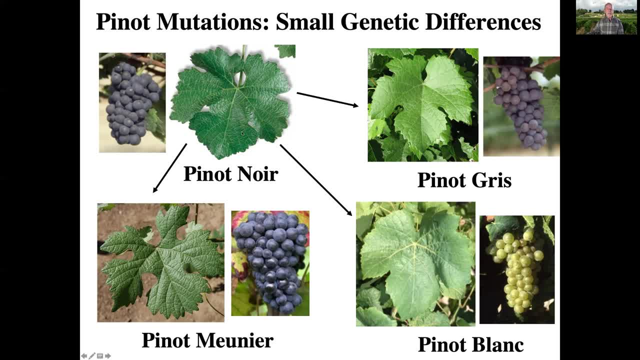 that causes this is a large difference. that causes this is a large difference in leaf shape and somewhat differences in leaf shape and somewhat differences in leaf shape and somewhat differences in the clusters. there have been other in the clusters. there have been other in the clusters. there have been other spontaneous mutations have occurred in. 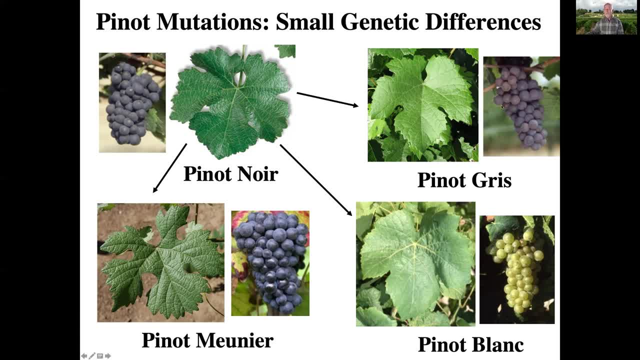 spontaneous mutations have occurred in. spontaneous mutations have occurred in the field that growers have identified, the field that growers have identified, which it'll led to the development propagation. so they have a mutation on a vine, they see it, they cut it off and they start propagating that mutation and 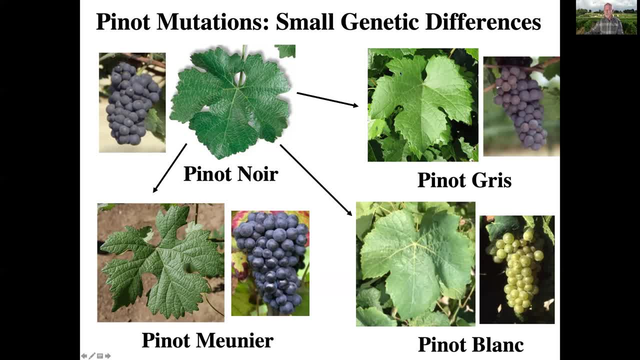 that's how these are generated. the same thing happens in apples, but in this case Pinot Gris has a lighter color in its cluster and often we make that as a white wine because we press it off the grapes very quickly to prevent the extraction of color out of the skin and again you can see the leaf shape is. 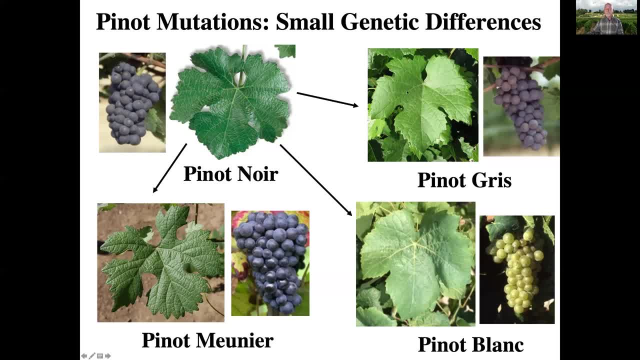 similar but has its own differences and unique differences. and again we have Pinot Blanc, a white grape that comes from Pinot Noir. so this is a mutation in a transcription factor that affects the synthesis of anthocyanins and it knocks it out and it no longer produces red color in. 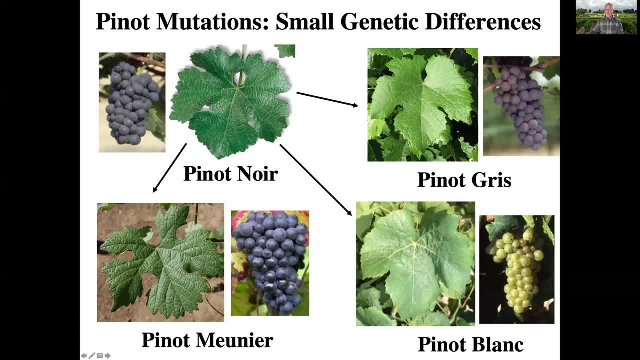 the grapes but only produces a green color or white white grape, and this has happened many times and other grape varieties as well over the years, as independent mutations that have knocked out this particular transcription factor that affects the biosynthesis of anthocyanins. but you can see that leaf. 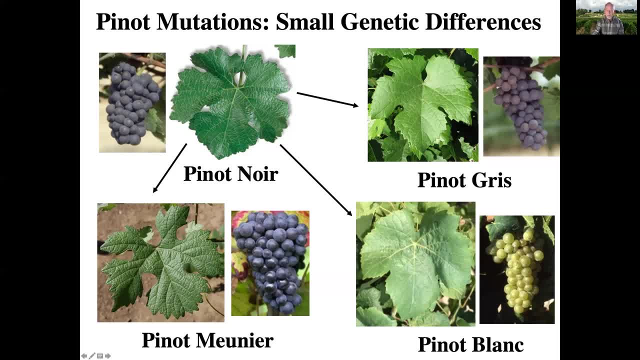 shape is also affected. so there are many, many genetic variations as a result of these mutations. There are many, many genetic variations as a result of these mutations. Remember, grape breeding does not produce consistent genotypes, so we have to vegetatively propagate the grape that we want, because the grape itself 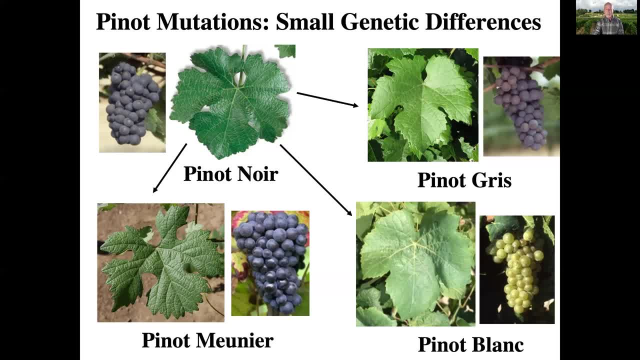 the genome is too heterozygous and we won't get the. if we cross Pinot Noir with Pinot Noir, we will not get the Pinot Noir genotype out of those seedlings. So the definitive way to identify grapes is to identify them in a variety of ways. So 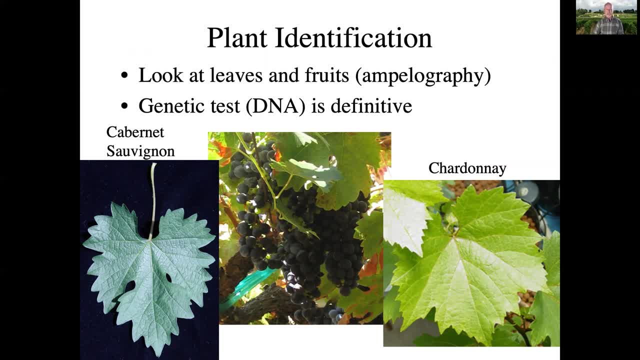 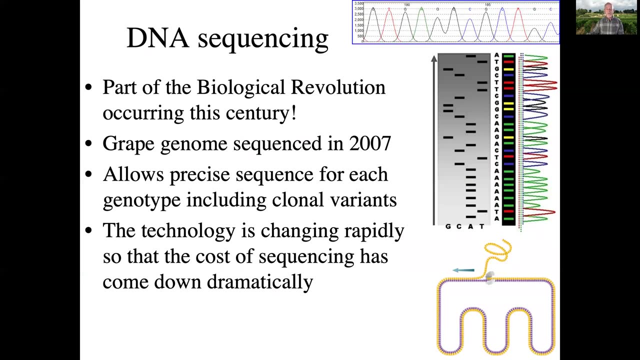 we have to get our DNA into the grape that we want, Which is much more consistent and accurate, is to use DNA testing that we have today. So this involves DNA sequencing as well, and this is a revolution that's going on right now in this century. It's 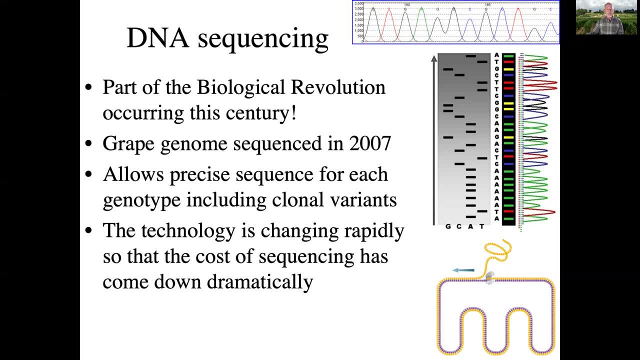 really contributing to our fundamental and deep understanding of biology. The grape genome was still was first sequenced in 2007.. There have been many other now great varieties like Cabernet Sauvignon, which I had a part in, that have been sequenced It. 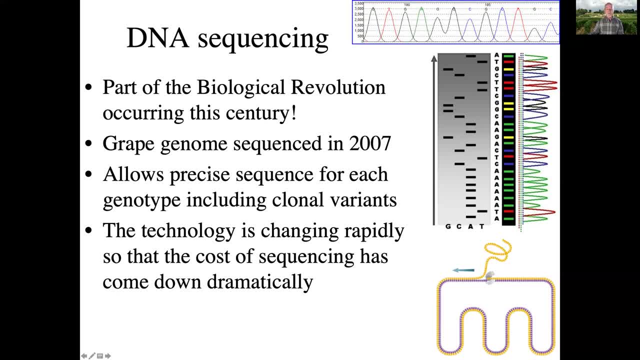 allows for understanding what the precise nucleotide sequence is for each genotype, including any clonal variants. So clonal variants may only have a single nucleotide mutation, or what we call SNPs, or single nucleotide polymorphisms that cause variation in the size of the 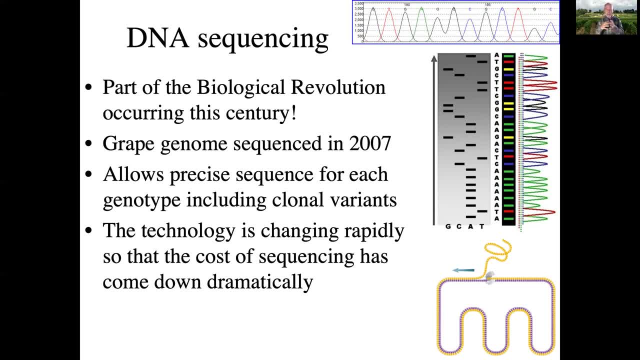 cluster, or the density or compactness of the of the cluster, whether it has wings on the cluster or not. There are lots of variations that go on in clones that still make it the same cultivar. The second variant is called the DNA. This technology, this DNA sequencing technology, has been changing very 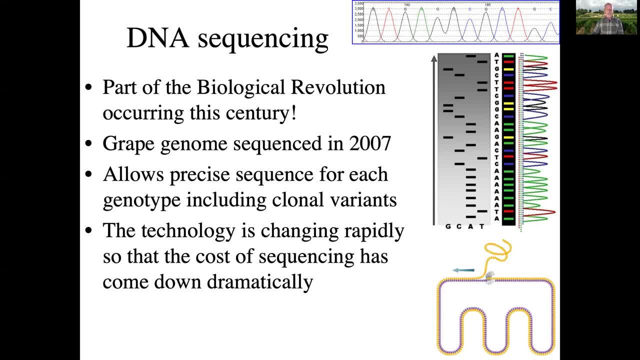 rapidly, and so the cost of sequencing has come down dramatically. Pretty soon you'll probably be getting your own DNA tested. I've already had mine done. I've had my sequence done, and it will be used for medical uses in the future for a. 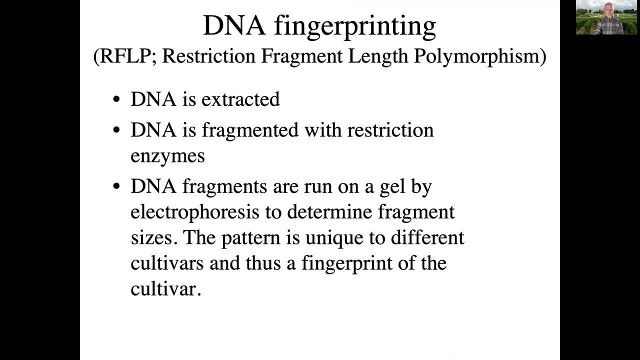 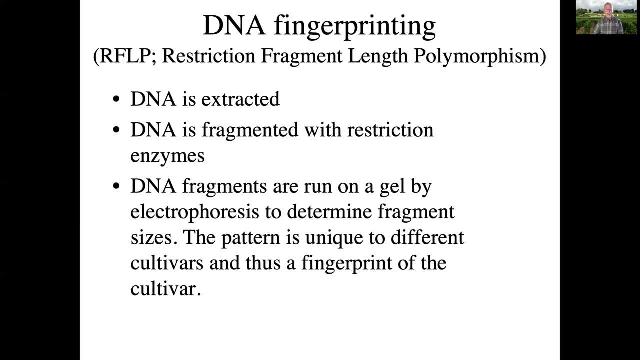 complicated group of devices. So I many, many, many PEs people are interested in- if you may give me just two seconds- when a CNClocally will be today- might introduce you to a genotype means And again you'll see. 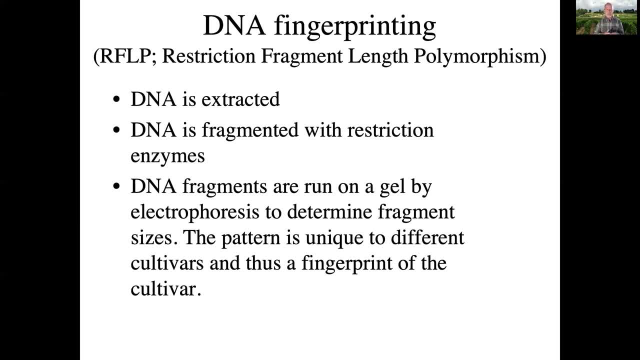 that often if you look at bracket fitting, you might see a- you know- coronavirus in the VR, which means it blood-like eczema unbundling um tumor You may also also be interested in, I would say, if Kinderman. 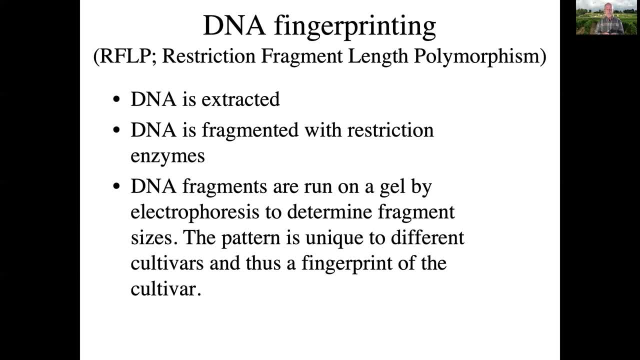 gets difficult. you want to take intome things right. Illecultrin, so that know whether it's sperm funding. embryoemo acre, embryoico Link, Italians, In other words, when your DNA is going to begin to. 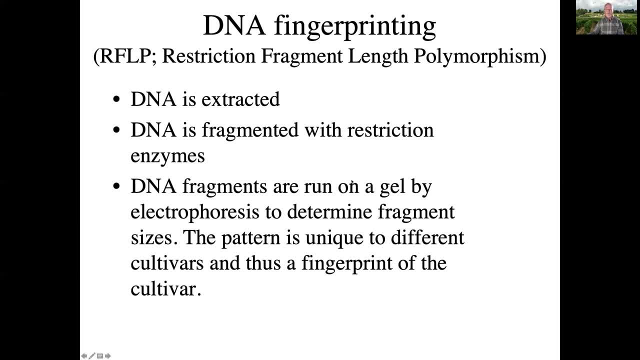 become what I calließ a precursor to sort of being inse 코로. one of our these fragments can be run on a gel by electrophoresis, a type of technique that moves those sequences by size through the gel, and the pattern is unique for each cultivar. 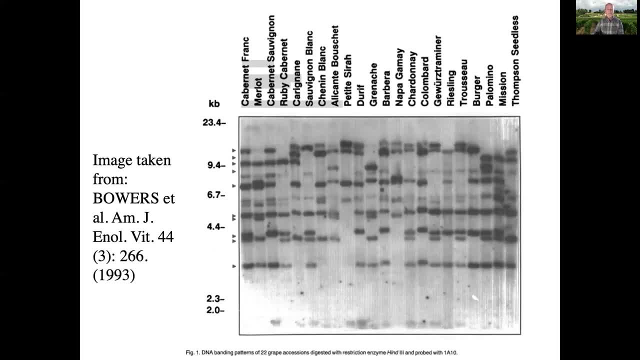 and thus we have what we call a fingerprint of that cultivar. here's an example of that, on which we have different cultivars along the top here and we can stain the dna and we can see the fragments. links are similar and some genotypes and different and others. 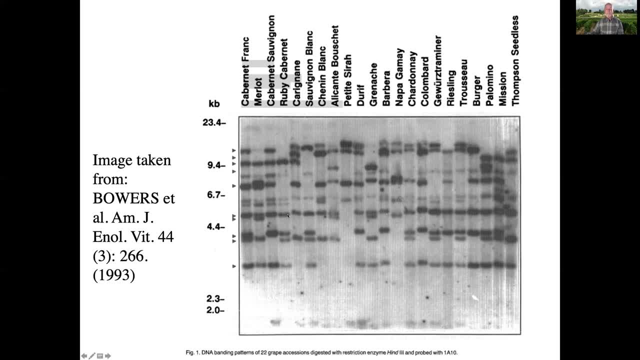 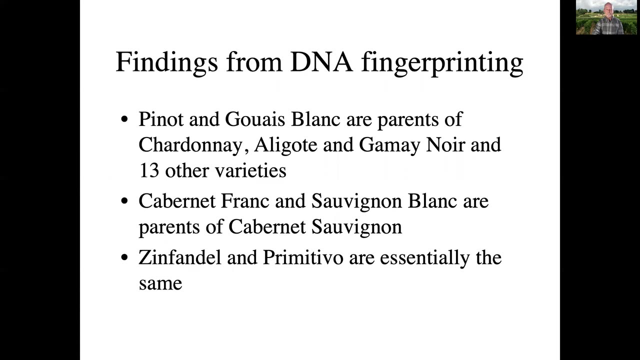 and you can line this up just like a fingerprint and identify what the cultivar is. unfortunately, it does not distinguish clones very well, and so this method really can only be used to distinguish cultivars which we can recognize in general. such findings have led to some interesting understandings, so for 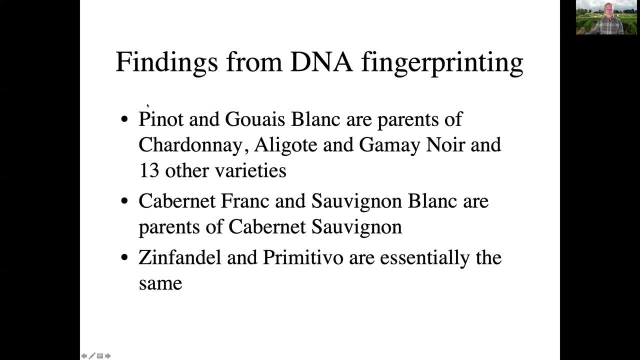 example, chardonnay comes from two parents: pinot, or pinot noir, and gui bon, which was considered a poor quality grape in france, and so the prestigious chardonnay came from a lesser quality parent, which was shocking to the french when this was discovered. 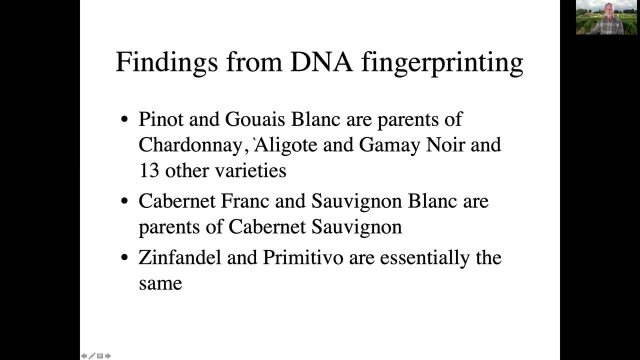 and Guy Blanc have given rise to other genotypes as well. Oligote and Gamay Noir and 13 other varieties have come from this spontaneous crossing in the field. So this was not deliberate work done by breeders, This was just spontaneous discoveries. 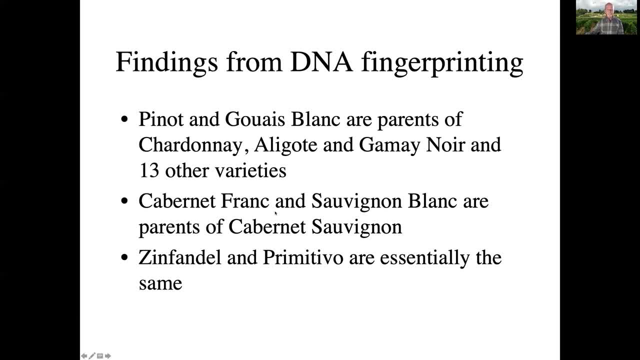 by people out in the field. that happened naturally And remember. pollination can be a self-fertilization of the flower, but wind or insects can also carry pollen to other genotypes and cause spontaneous or natural cross. Another interesting discovery was that the parents 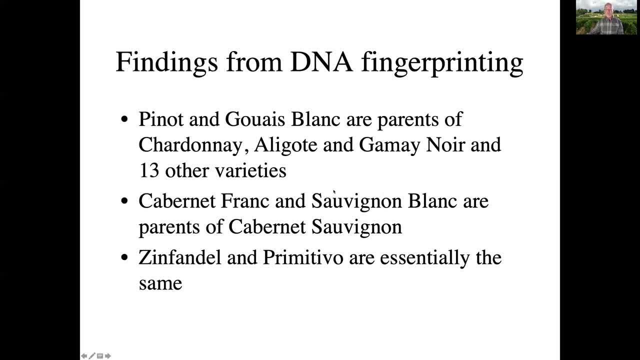 of Cabernet Sauvignon are Cabernet Franc and Sauvignon Blanc, And this is again a natural occurrence that occurred in the fields in Bordeaux somewhere, And then finally, through a sort of genetic detective test, it was discovered that Zinfandel actually originated. 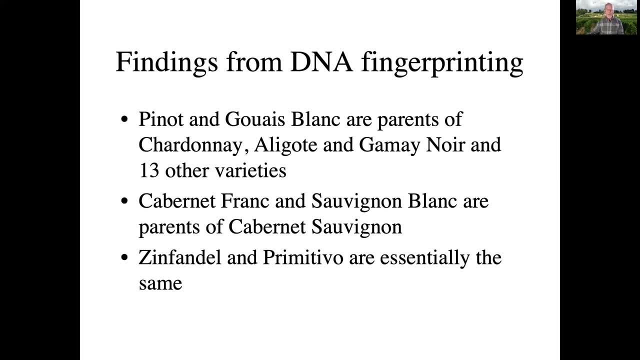 from Croatia and was carried down to Southern Italy, where it was then brought to the United States, And the grape variety that we call Permitivo is essentially the same as Zinfandel. Some people call it a clone and some people call it a home of Zinfandel, or vice versa. 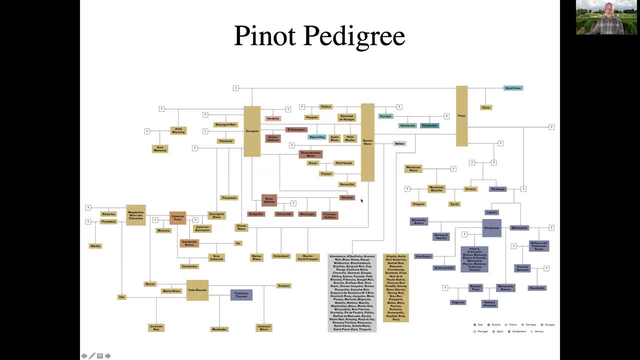 Here's just a map. I don't expect you to see this or understand it, but it's a map of the Pinot pedigree as determined by geneticists using this technique. So there are lots of different genotypes arising from this original parentage. 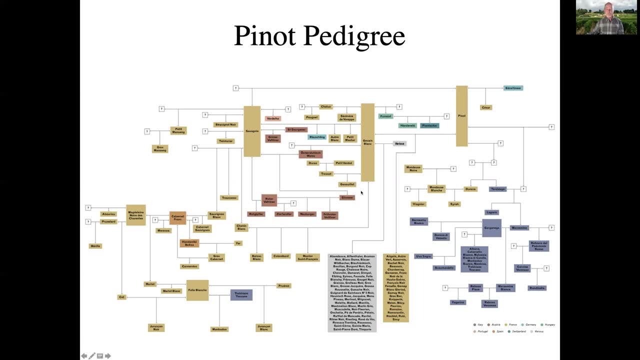 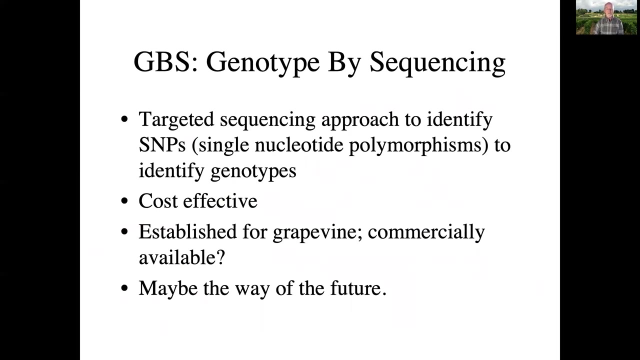 and gives us the diversity that we see. There are over 7,500 different grape vine genotypes today, and it continues to grow. So finally, in this last slide, I just want to talk about a futuristic technology that's here today, and this is called GBS for short. 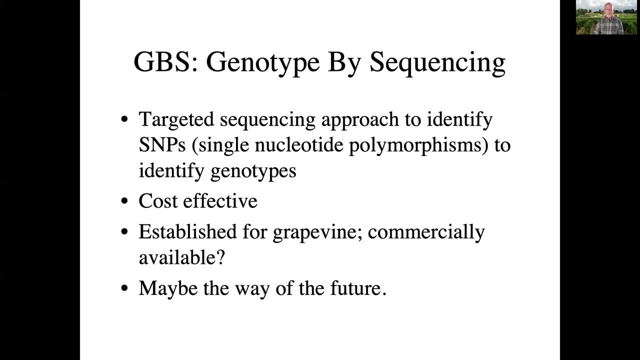 or genotype by sequencing. It's a targeted sequencing. So we're sequencing the nucleotides, but we're only sequencing certain parts of the genome rather than sequencing the whole genome. This makes it more cost effective, And what we're looking for are these single nucleotide polymorphisms. 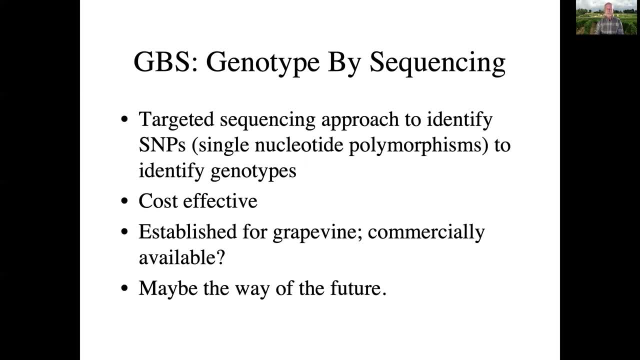 just a single difference in a nucleotide sequence that is specific to a clone or a cultivar to identify the genotypes. This methodology is being established and has been used to identify grapevines. I'm not sure that it's commercially available at this point in time. 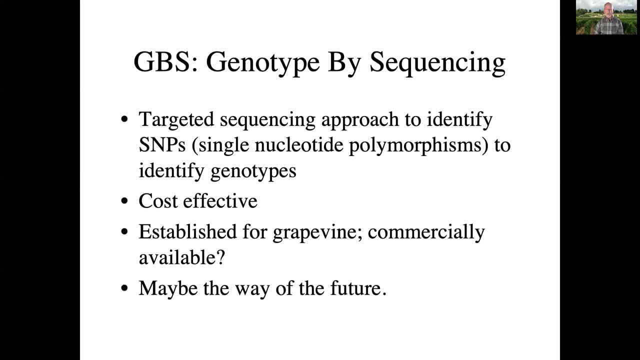 but I expect it will be in the future. So I hope you found this talk informative and you go out now and look in your vineyard at the leaves of your grapevines and look at the variation on a single vine and or look at variation and leaves between different vines. 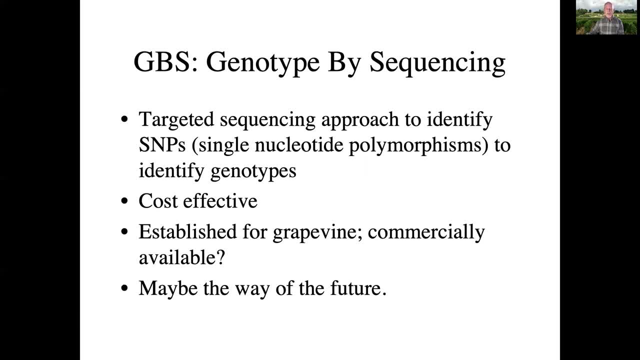 And know that if you really really want to know what grape variety you have, you need to have your DNA sequenced and identified for that genome. UC Davis does perform that methodology and can identify your genotype. if you're concerned, I am not sure what the cost is.